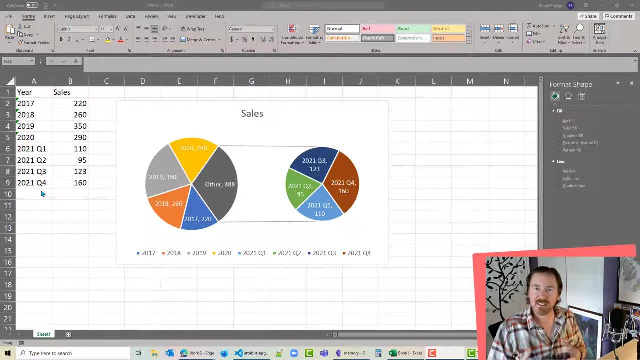 2021 into four quarters and I want to kind of illustrate that in a chart So you can see. I've got my pie wedges for the main sales chart here, but 2021 splits up into its own little pie chart. I'll click anywhere in the chart area. 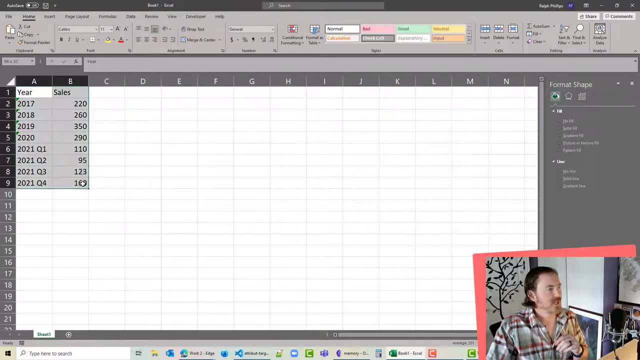 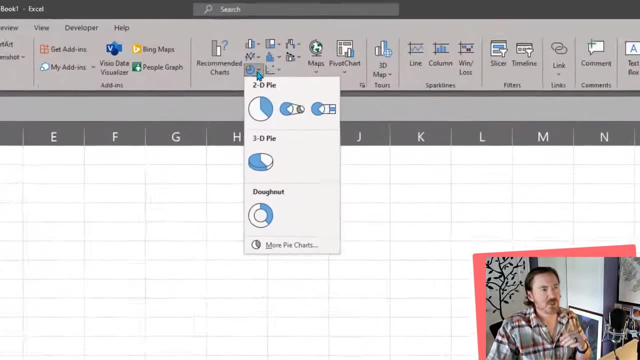 delete that. let's give it a try. So I'm going to go ahead and select my sales data just as I would making any other chart, and on the insert ribbon head over to the pie chart area and I'm going to choose the option here: pie of pie and. 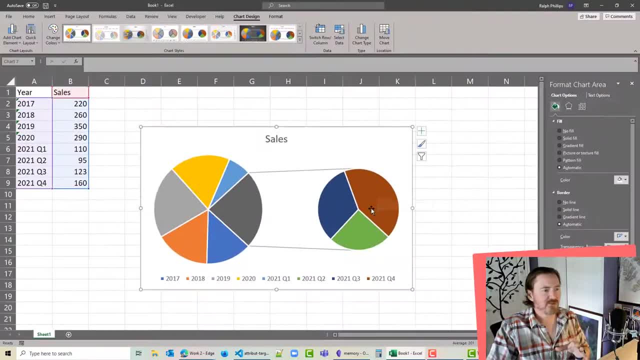 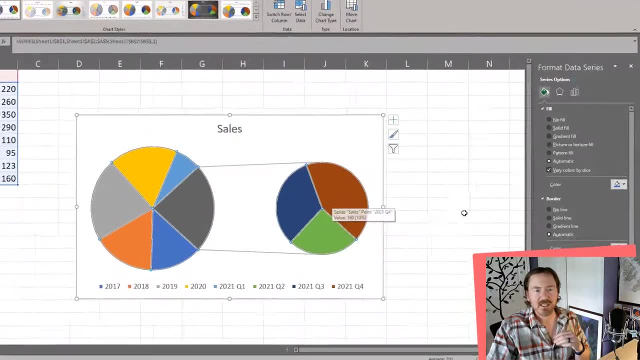 I'm going to click on that Now. by default, it's only showing me three options here. However, I can click anywhere to select that pie of pie and click on that. I'm gonna get some options over here on the far right and under format data. 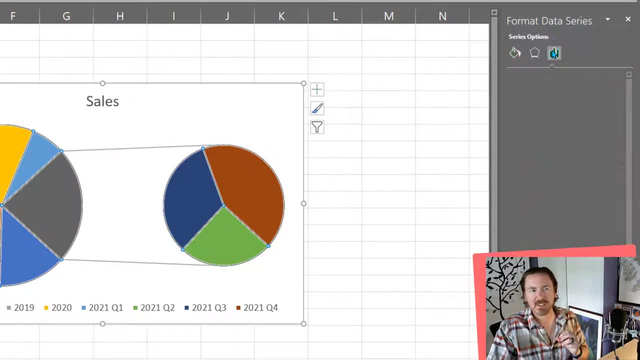 series. however, I want to click over on the series options and under the series options I do see this values. in my second plot it's set to three. now if I went down to two or one, which would be kind of silly, that's not what I want. I'm. 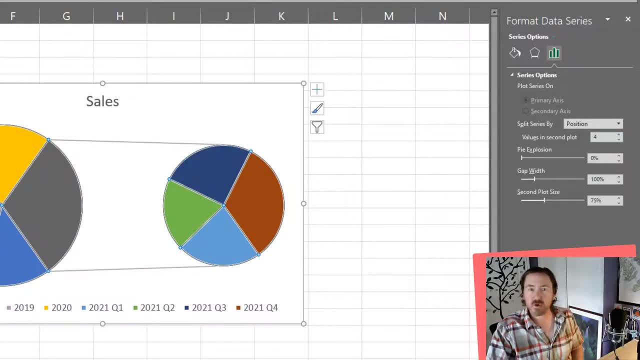 gonna move it up to four because there are four quarters in that total series that I want to show. so now my PI wedge, my PI wedges for this PI of PI. you'll see that I've got the light blue, green, dark blue, rusty orange there and that. 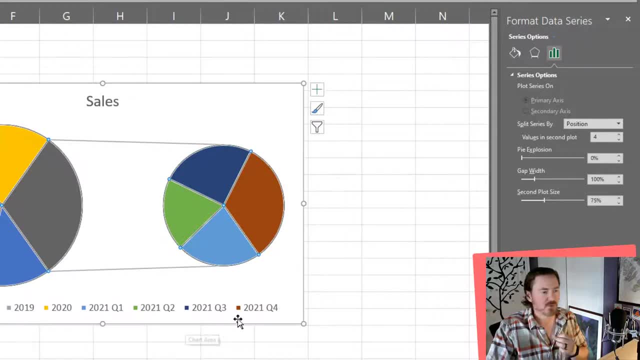 corresponds down here with twenty twenty, one quarter, one quarter, two quarter three and quarter four. great, so that's how I can do that. now you can play around also with the second plot size. currently it's 75%. if that was 100%, then both of these pie charts are going to be the same size. 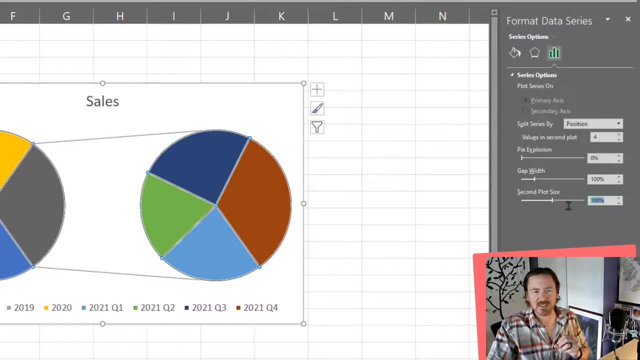 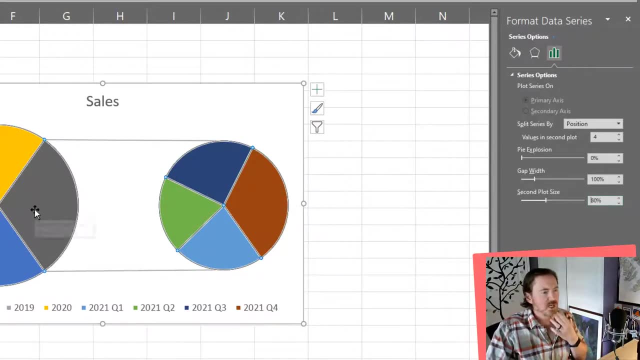 however, I can kind of like it when the second pie chart is up just a little bit smaller, because it makes it clear to your audience that this second pie chart is more of a subset of the primary pie chart, and that's a lot of PI wedges to. 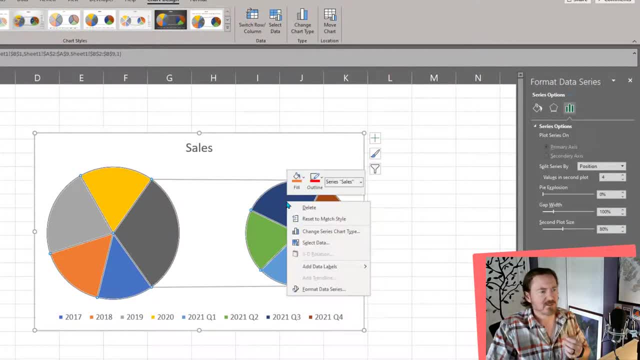 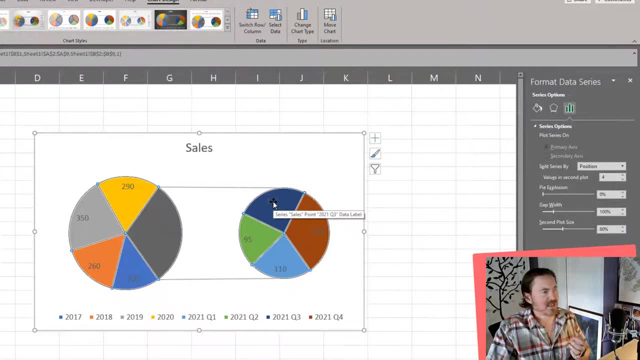 look at. so while I'm here, actually I'll just right-click on any one of these PI wedges and I can add data labels, pop those in there. then I can right-click on any of those data labels and choose format data labels and that'll customize. 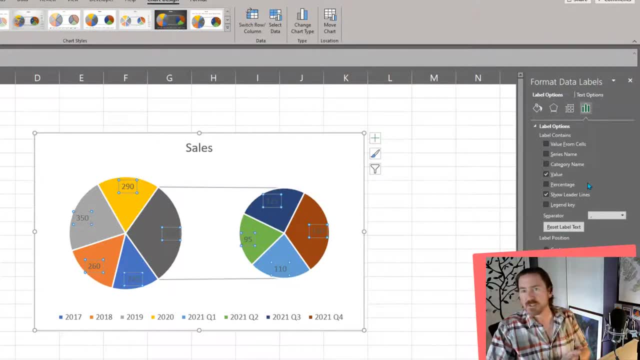 my format pane to show those. and let's see, you can see that I've got a lot of pie wedges and I've got a lot of pie wedges. you know what? to make these really easy to see. while they're all selected, I can go back to my home ribbon and just choose a nice white font, since they all 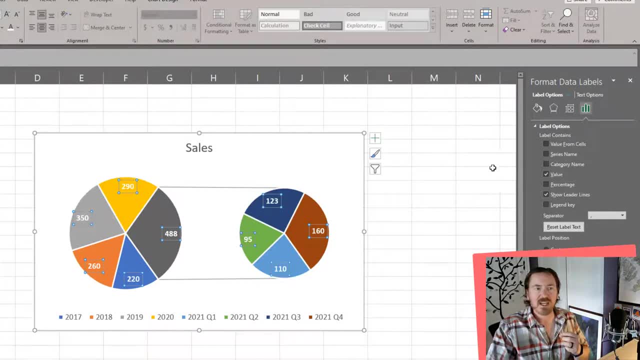 seem to have kind of dark backgrounds, I'll make those bold as well, and then back over my format data labels. let's see, I think values still look pretty good, but maybe I'll choose the category name in there as well. then you could play around with those as you need to, but once you feel like you've got it set, 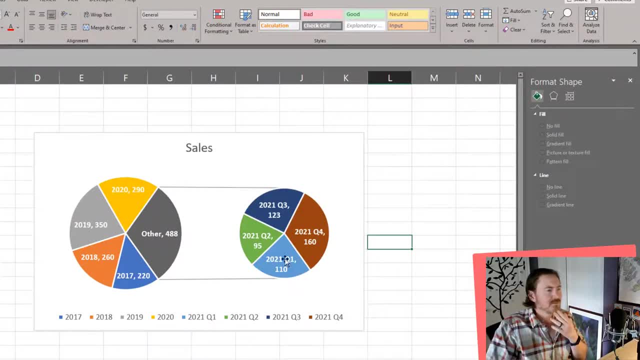 up right, you've created your pie of pie chart, so now I've got for the main pie chart. off to the left, I've got 2017, 18, 19 and 20 and then, although it's labeled as other, that's our 2021 pie chart, which leads over to this right side. 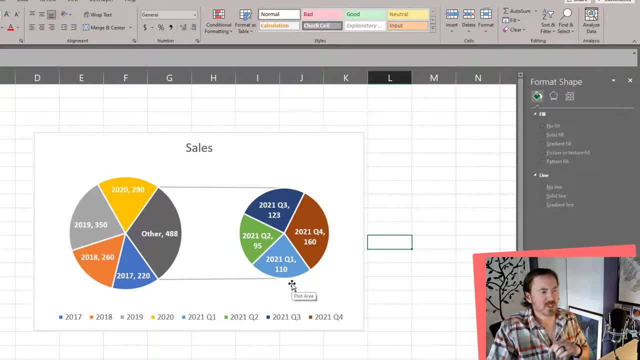 pie chart where I can see each individual quarter of 2021 and start to appreciate the impact of the sum of all of those and with the main pie chart. but we do want it to be clear to our audience what's going on here. so, if I 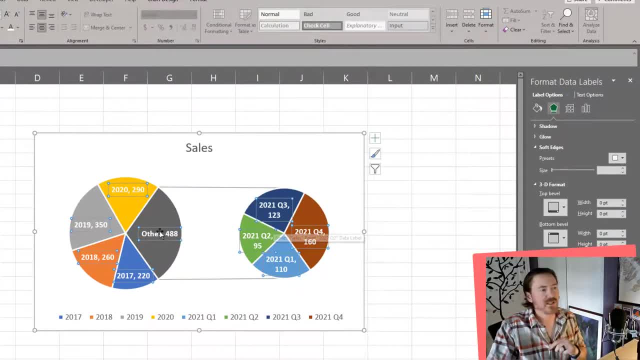 click once on any of these data values, notice they all get selected. But if I click once more on the other comma right there, I can actually edit that one right there And I'm going to go ahead and change it out to 2021. 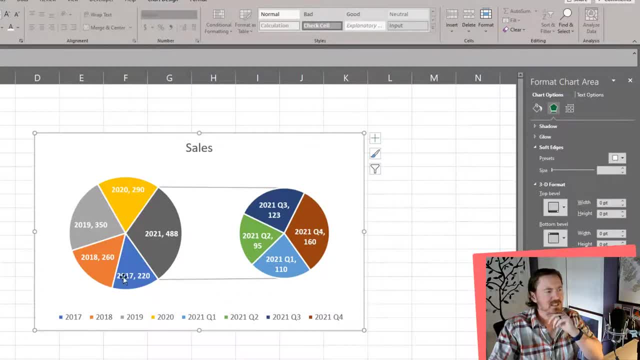 Everything else is going to stay the same. So now it really stands out which years are involved, And I can see, just by looking on my left pie chart, that 2021 is a bigger pie wedge than all of these other pie wedges. And now for the real details. we can say: well, what was going on in 2021??